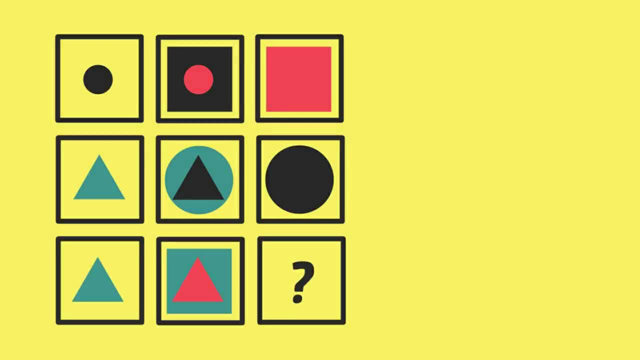 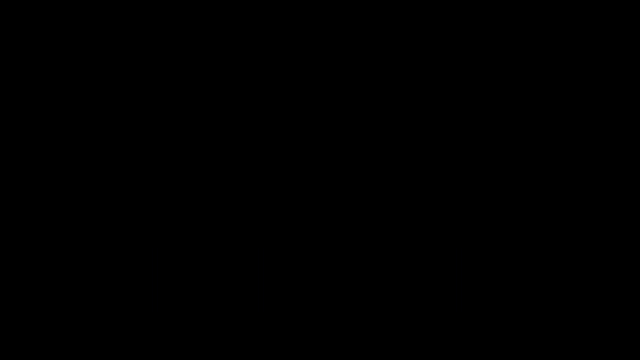 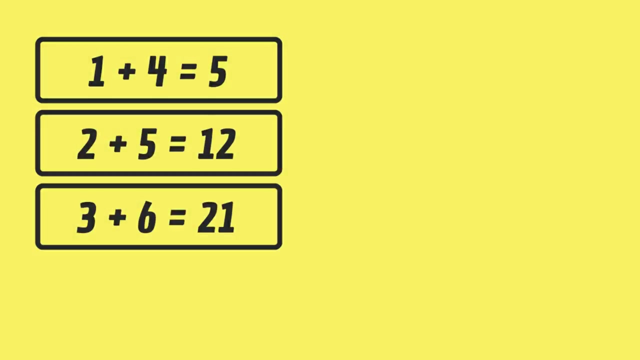 For one. the best choice to complete the last pattern is A, B or C. Well, the answer is B. the pink square Question number two: If 1 plus 2 equals 5, and 2 plus 5 equals 12,, 3 plus 6 equals 21,. 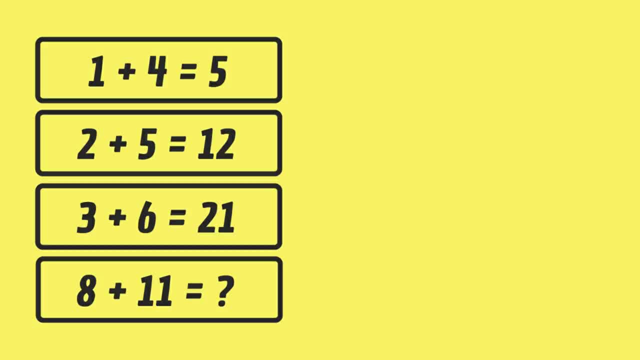 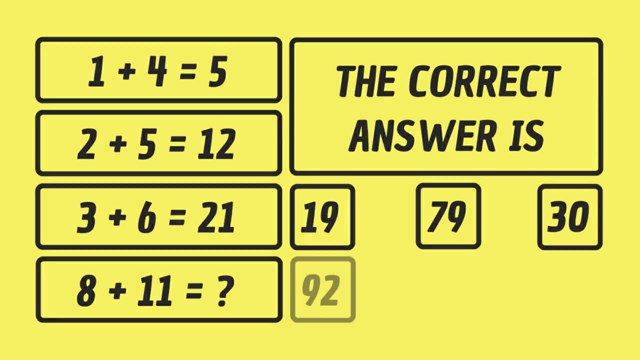 then 8 plus 11 equals. The answer is 19,, 79,, 30,, 92,, 96, or 100.. You have 15 seconds For one. the best choice to complete the last pattern is A, B or C and 2 plus 5 equals. 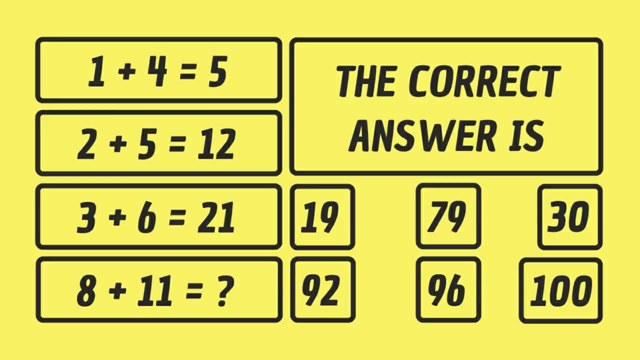 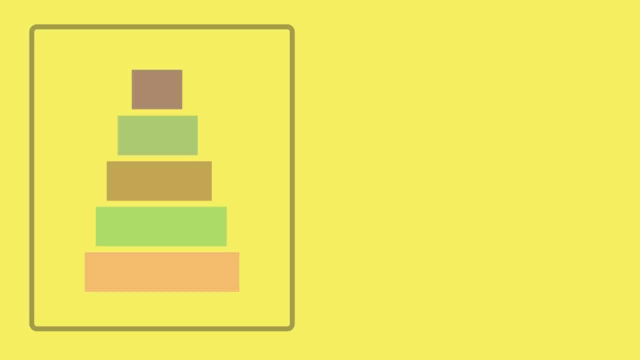 5, and 2 plus 5 equals 12,, 30,, 92,, 92,, 92,, 93, or 100.. You have 15 seconds. The answer is 96.. Question number three: If we see the pattern from above, what does it look like? 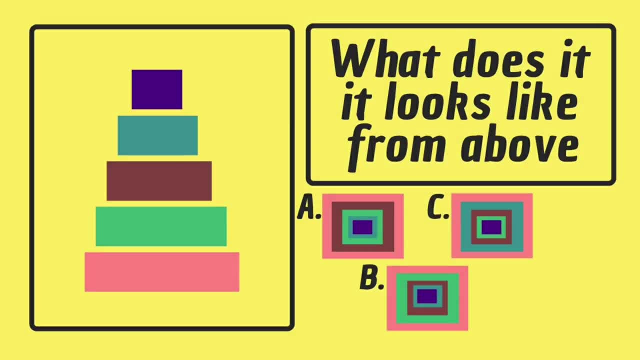 A, B, C or D? Question number three. If we see the pattern from above, what does it look like? A, B, C or D? Question number three. If we see the pattern from above, what does it look like? 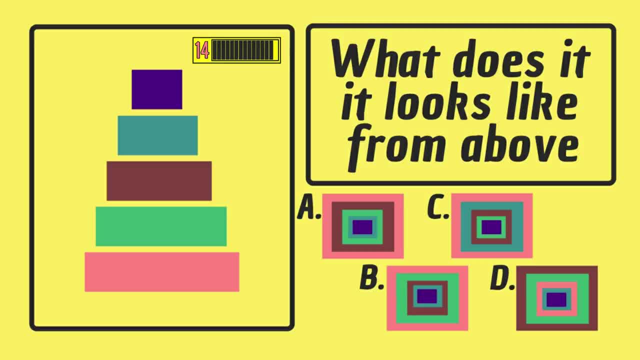 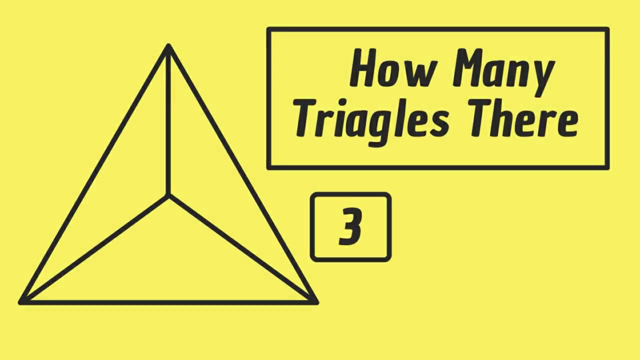 A, B, C or D. The answer is B. It's purple, blue, brown, green and red. Question number four: How many triangles there? 1,, 2,, 3,, 4, or 5?? 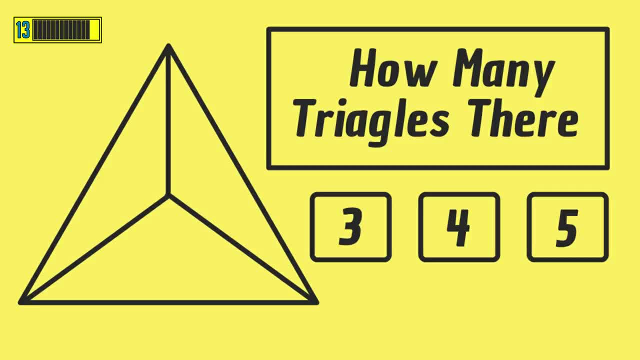 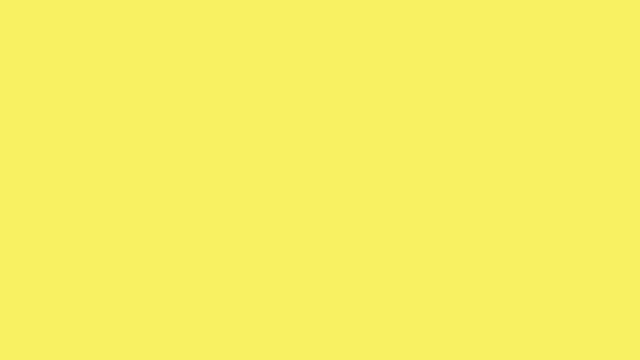 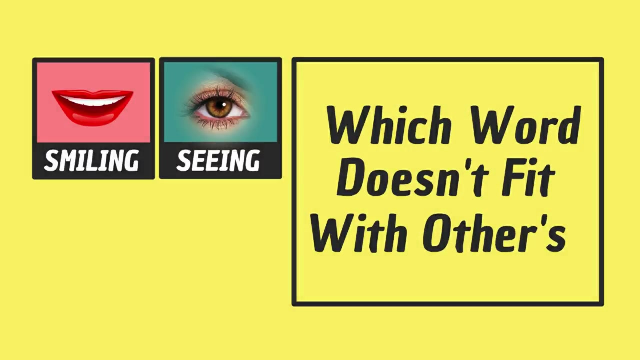 3,, 4, or 5?? The answer is 4, with three small triangles and one big triangle. Question number five: If we see the pattern from above, what does it look like? 5. Which word doesn't fit with others? Smiling, Seeing, Hearing or Smelling. 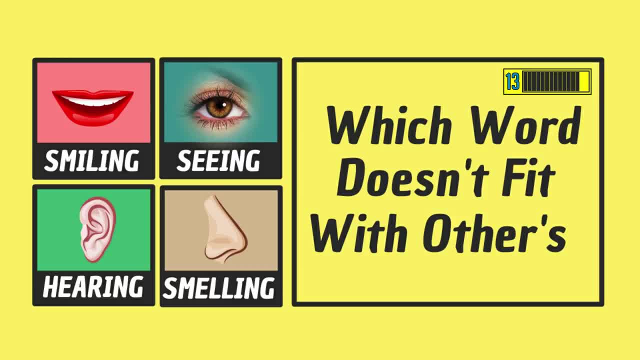 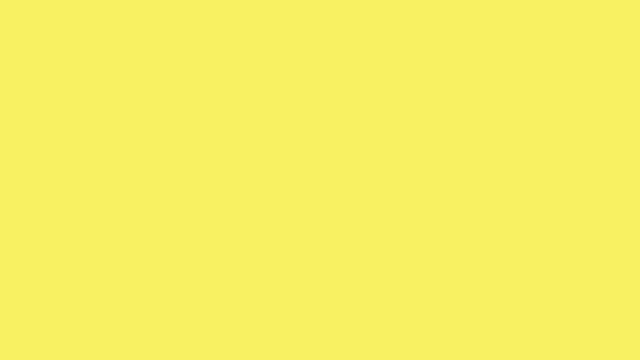 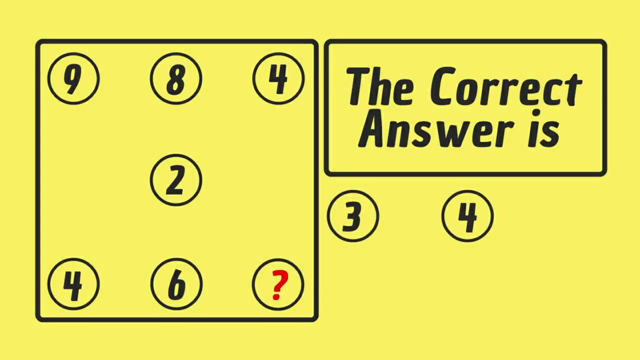 Yup, the answer is smiling. It should be talking instead 6.. The correct number to fill the question mark is 3,, 4,, 5,, 6,, 7, or 8?. The answer is 7.. 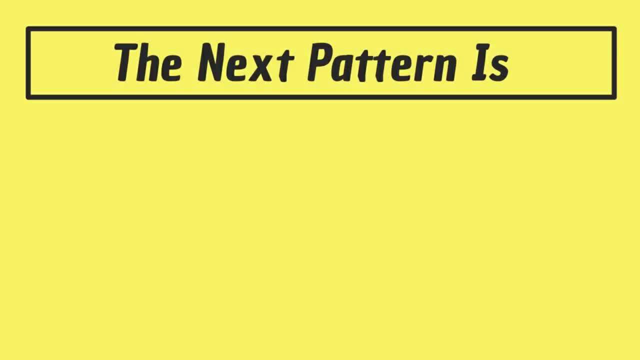 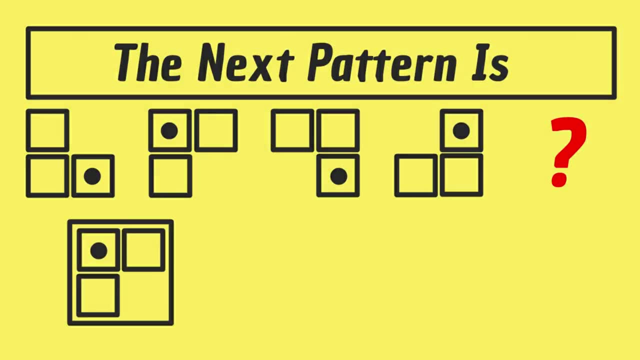 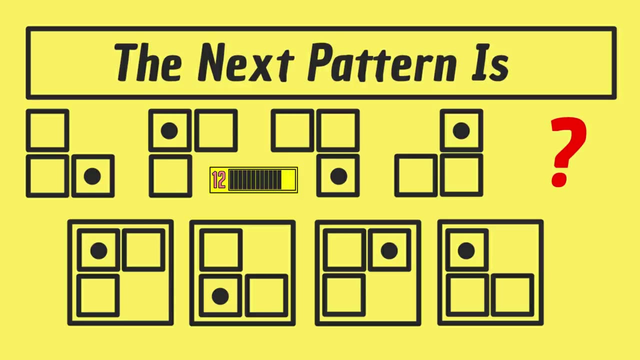 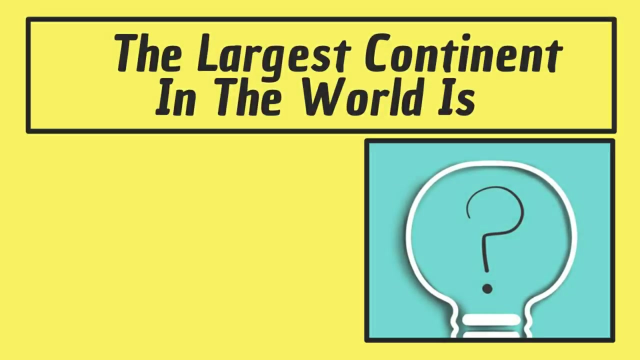 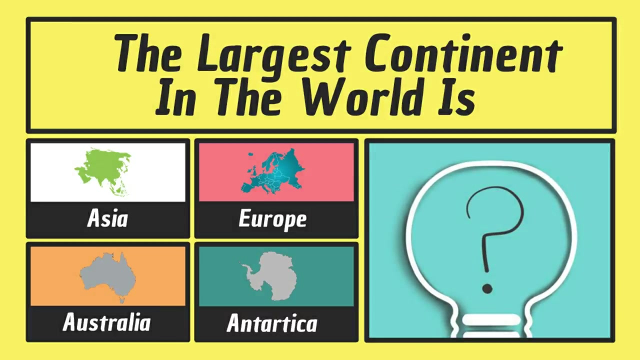 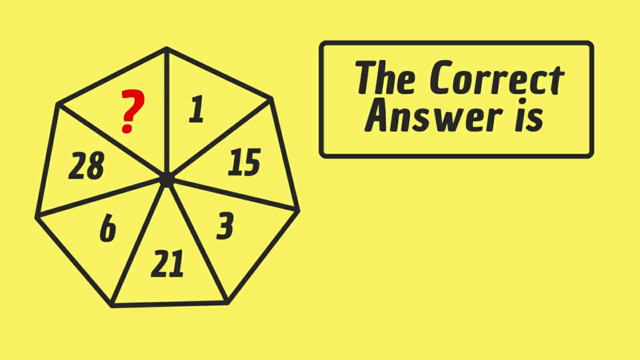 Question number 7.. The next pattern is A, B, C or D. Correct, it's B, Question number 8.. The largest continent is Asia, Europe, Australia or Antarctica? Well, it's Asia, Question number 9.. The correct number to fill the question mark is: 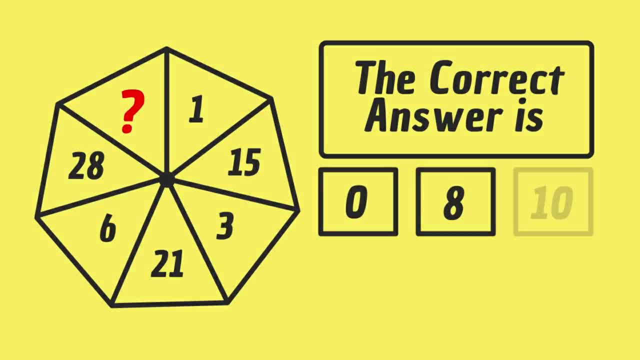 0,, 8,, 10,, 13,, 29, or 36? Correct, it's C: 5,, 6,, 5,, 6,, 7, or 10?. 5,, 6,, 5,, 6,, 7, or 15?. 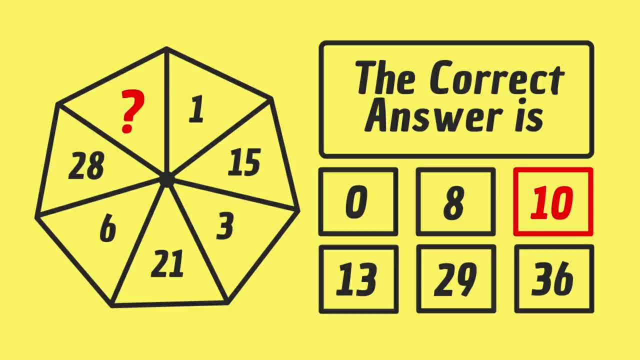 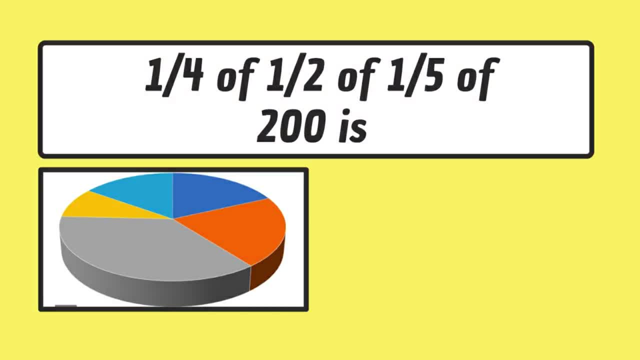 The correct answer is C, The last 1 guys, Question number 10.. The correct answer is 2,, 4,, 5,, 10,, 25, or 57?? Okay, Let's do it again. Press it. Yes, one, 2,, 4,, 5,, 6,, 7, or 18?? Question number 15.. donuts Three, two, 1. 5.